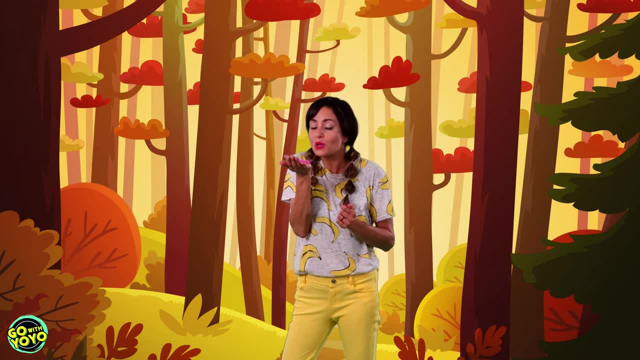 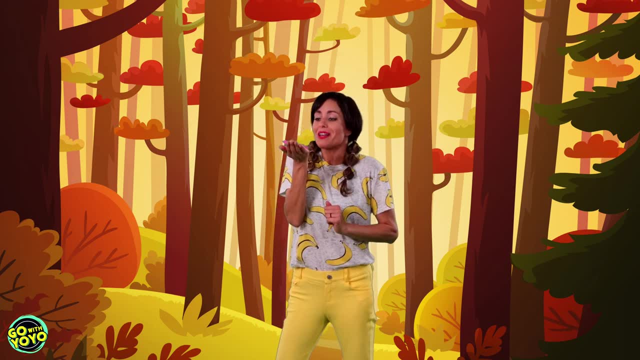 And I'm going to blow really soft in my feather so it doesn't blow off with my hand. Maybe we can try a really hard breath Ready, Take a deep breath in, Breathe really hard. It fell away. Now let's see if we can do it again, and this time let's not. 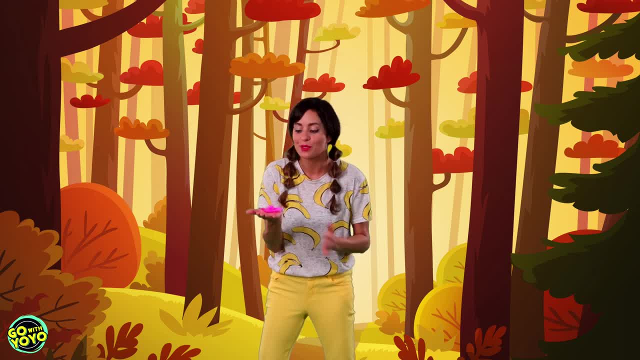 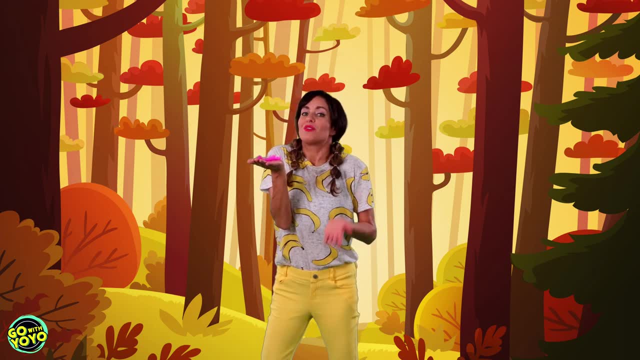 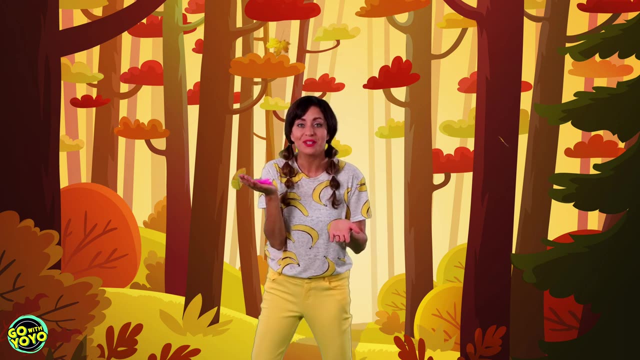 Let's not breathe so hard. Let's breathe really slow and calm, so the feathers don't blow off my hand. Are you ready to try it? Okay, here we go. Breathe in through your nose And breathe really slow. That's it. They didn't blow off. Let's do this again. 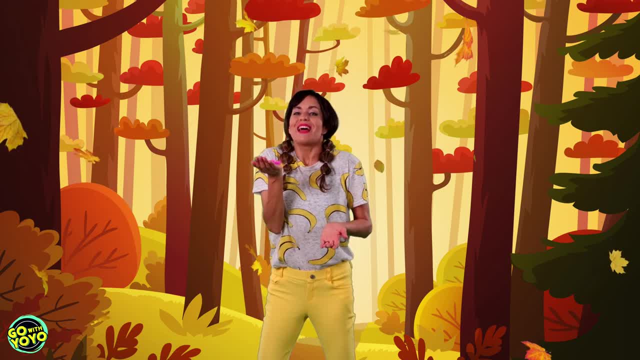 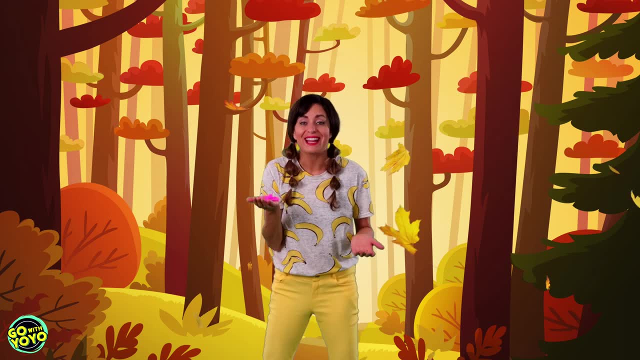 Breathing in through our nose- You got it- And then breathe out real slow out through your mouth- Ready, That's really great. Let's try it again. This time we're going to breathe only through our nose. Let's see, I wonder, will the feather blow off? 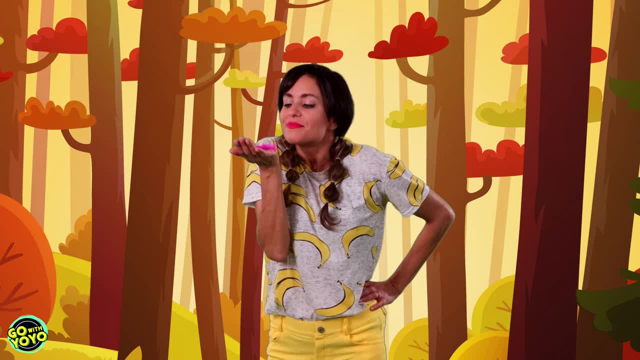 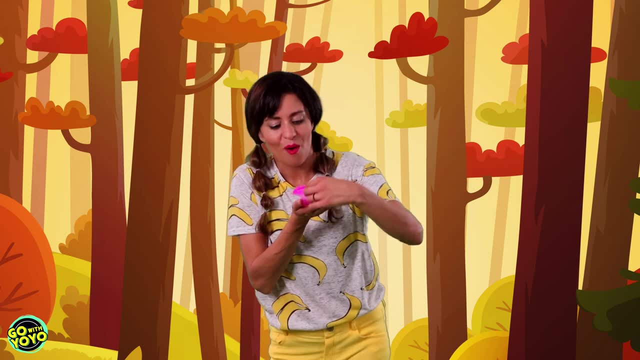 Okay, let's try it together: Breathe in through your nose And out through your nose. Oh no, It almost fell off. Wow, Let's try it again. Let's breathe in through our nose and out through our nose. 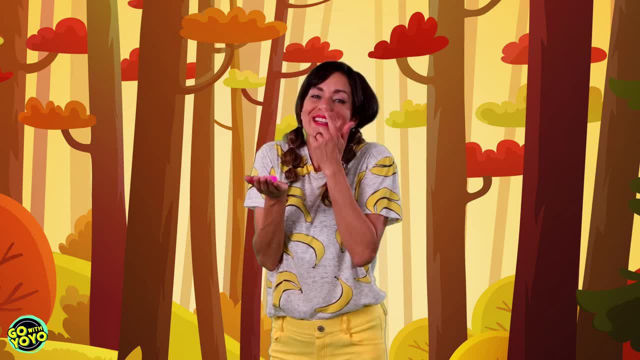 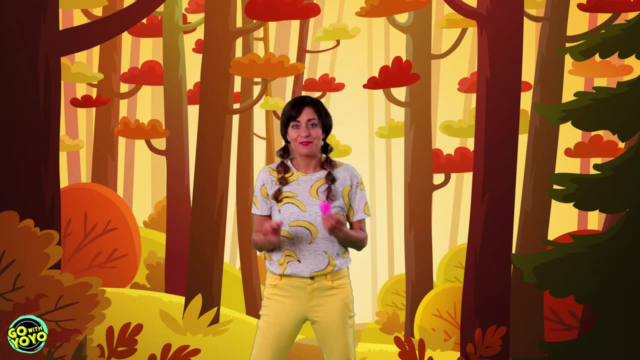 You're doing great Ready Breathe in And breathe out. Oh, it didn't blow it off at all. Now I'm going to try a really fun feather game with you. Now, if you have a feather, that's great, But if you don't have a feather, you can also use a tissue too. 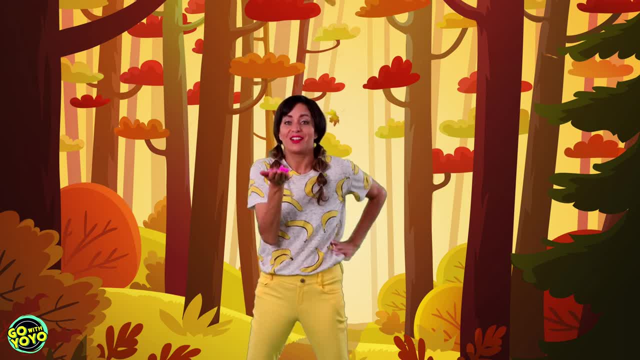 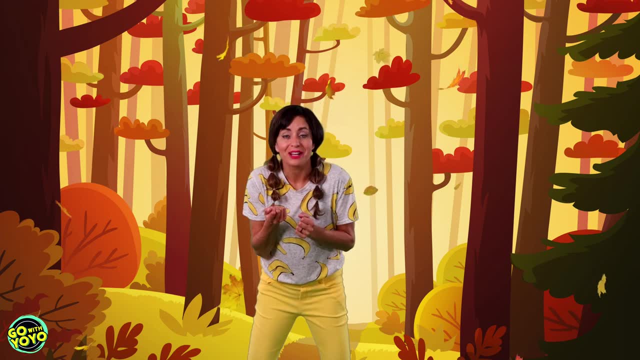 You can put that tissue in your hand. Let's try this together: You're going to take a deep breath in And we're going to blow the feather or your tissue off your hand And then you're going to try to catch it. Do you think you can do that with me? 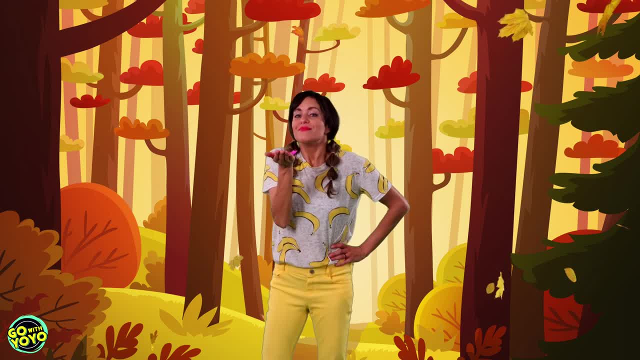 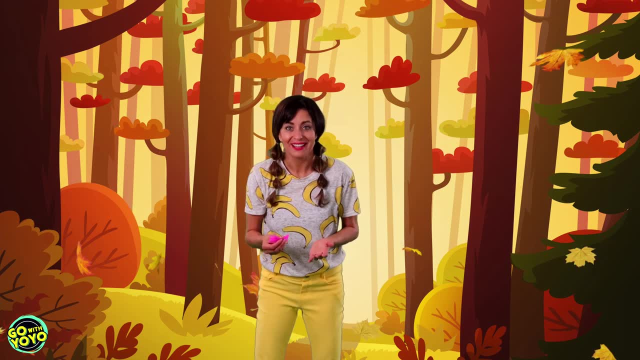 Okay, ready, Breathe in And blow it out. Oh, I caught it. And if we don't catch it, that's okay, We get to try it again, Alright, so we're going to put it on our hand. Here we go. 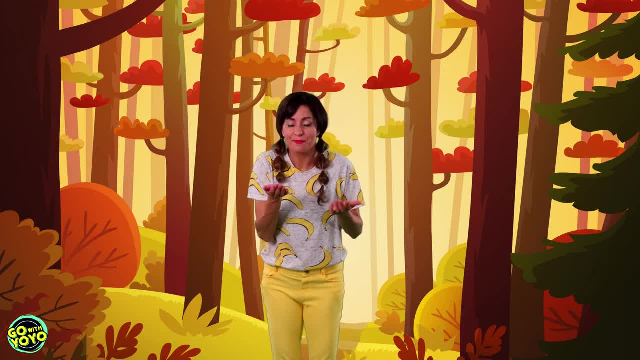 Take a deep breath in through your nose. That's it Ready And blow it out. Oh, and try to catch the feather. Wow, I caught both of them. Alright, friends, how are you feeling? I'm feeling a little bit calmer, a little more peaceful, a little more relaxed.